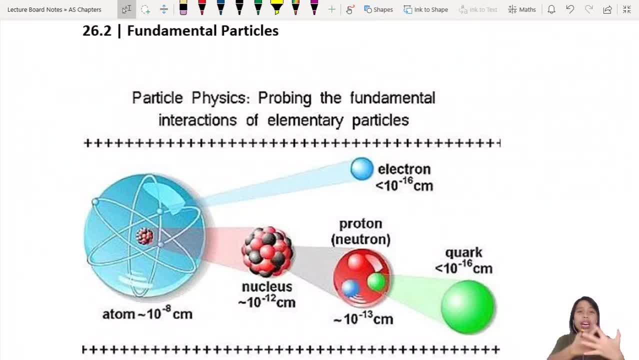 Hello, We continue our journey into the unknown, or at least it was once an unknown. So the story goes like this: Okay, we know our protons, we know our neutrons, we know the structure of the atom. It was a great time to learn about the nucleus. Okay, chemists and 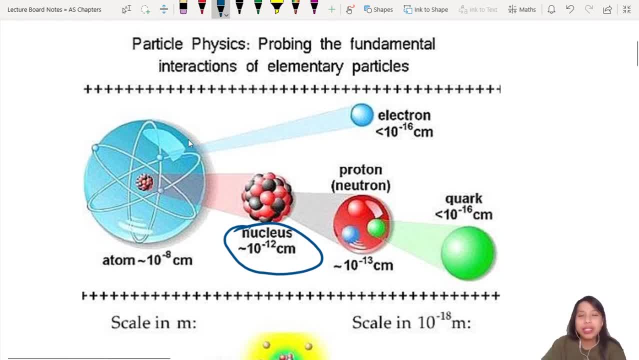 physicists were working together, making great discoveries. It was an amazing time to study chemistry Basically. you got a nice periodic table. you know the groups, you know the properties, you got names for a whole bunch of elements. People were very, very, very amazed and very. 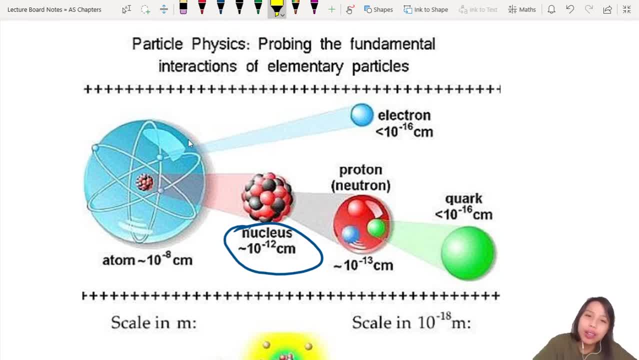 happy. At some point we, kind of the chemist, was like: um, I guess we're satisfied, we're fine, we got our table, we know our properties, It's more than we need to know, okay, But then the 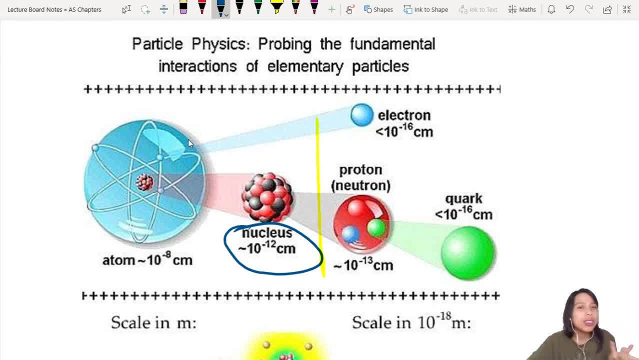 physicists were like: wait, wait, wait, wait, wait, but. but. but is the fundamental particle, the proton, the neutron? Surely there must be more than that. And so they were asking the question: are there any more? 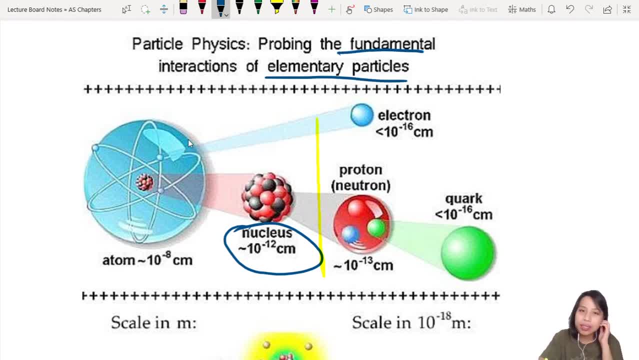 fundamental particles. Fundamental, or I guess you can say elementary particles, that is smaller than a proton or a neutron. And yes, you can see this picture here. They see like, okay, if you're a proton or a neutron, actually you can zoom in some more. and there's these three things here. What are these? 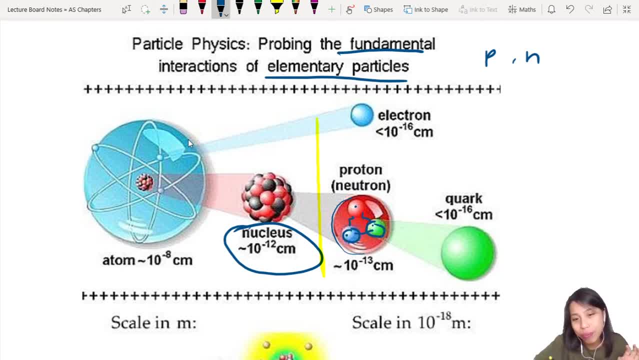 three things. Ah, that's what we'll look at today. Okay, these are what we call quarks. They're like: what are quarks? Well, they are just fundamental particles. That's why this section is called fundamental particles. So if you look in scale, 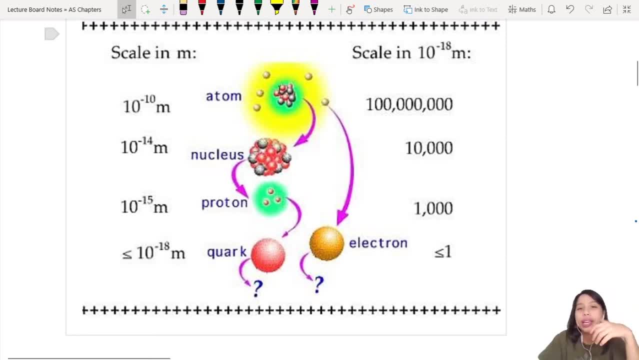 what we're doing is we're really zooming in closer and closer where chemistry left off and we're going where no man has journeyed before, Or, no, no science has journeyed before. So go smaller. zoom into atom. you get nucleus. Zoom into the nucleus. you have proton and neutron. Zoom into. 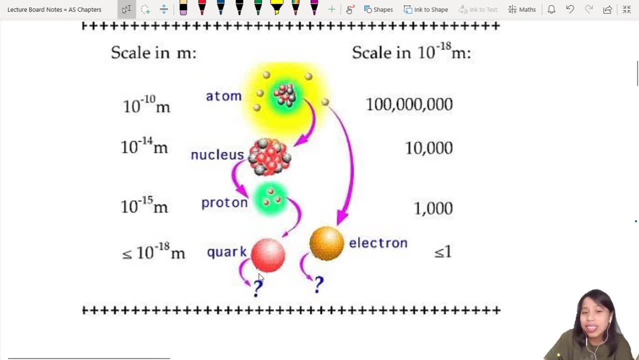 the proton, you get quarks and electrons. And is there anything smaller that? can we break down the quarks somehow? We don't know. Honestly, I don't know. If you discover this in the future, please win the Nobel Prize, okay. So anyway, how do people do this thing? 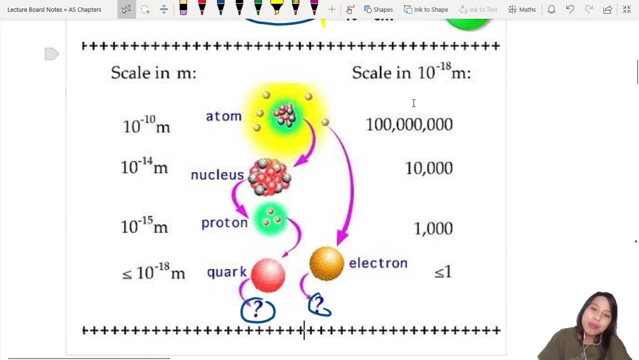 Well they were, I guess you could say, inspired by Rutherford's experiment. Rutherford's like: oh, I don't know what's inside, Let me shoot alpha particles in Pew, pew, pew, pew, pew And, I guess, as a habit that physicists have. you don't know what it is, you just shoot things. 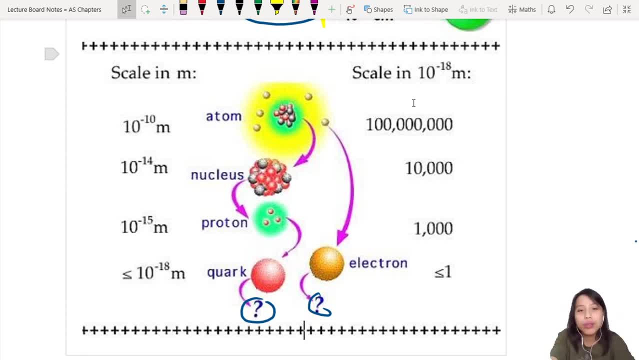 at it. Shoot things together to make them explode and see if you can see what's inside. You take a watermelon, you take a pumpkin, you throw together, you see the thing explode. that's how you study, okay. So they make things like these. 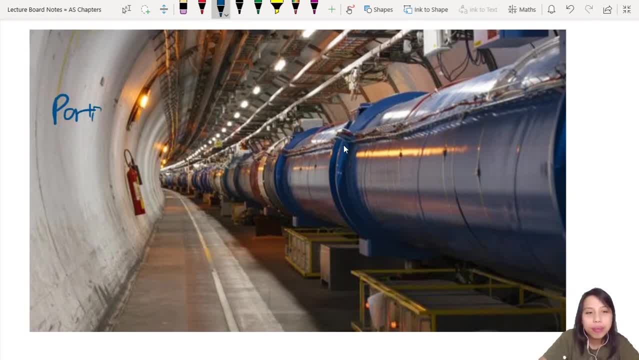 This is what we call a particle accelerator, where people use to study high-energy particle physics. You see this long blue tube, right Accelerator. Basically, the particles inside there are flying down the tube and it goes in the ring. We'll see more pictures later. okay, So they'll be. 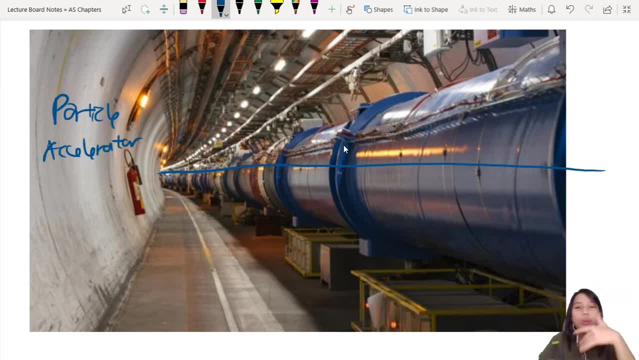 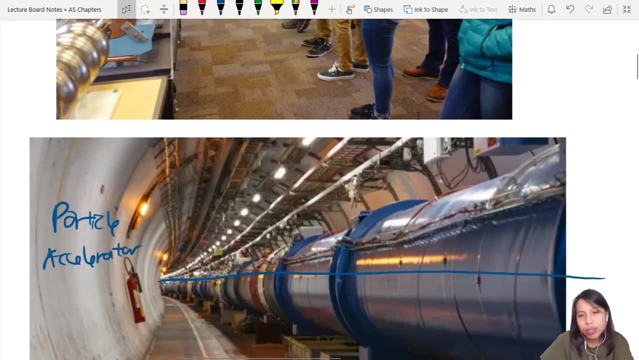 shooting together, I guess gold, nuclears or whatever element they choose to shoot inside there. okay, They'll speed it up with electric fields and things like that, And inside there it's kind of a hard picture to see. It looks something like this: You have lots of rings, There's only 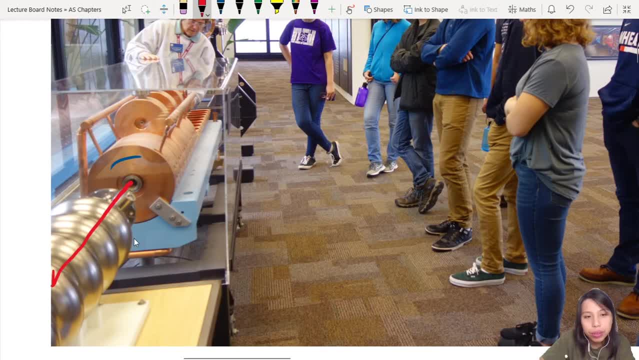 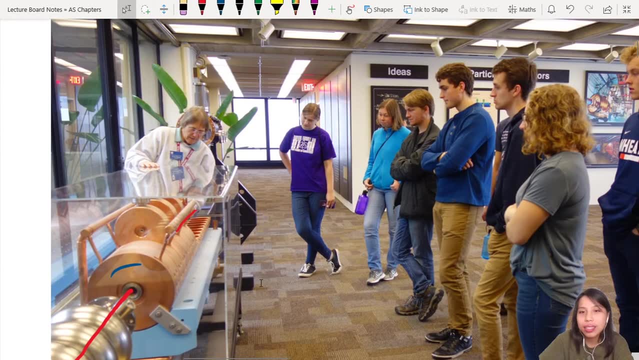 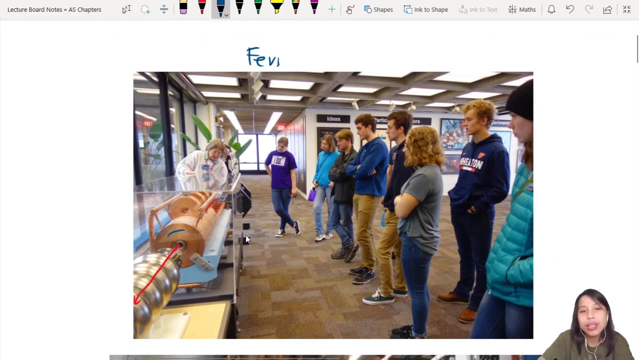 a tiny, tiny hole where the particle will travel through. So it's going in the middle of all these rings, which we'll figure out what we do. I took this picture, Nice right. We got to visit Fermilab, one of the premier areas, old place where they first started. 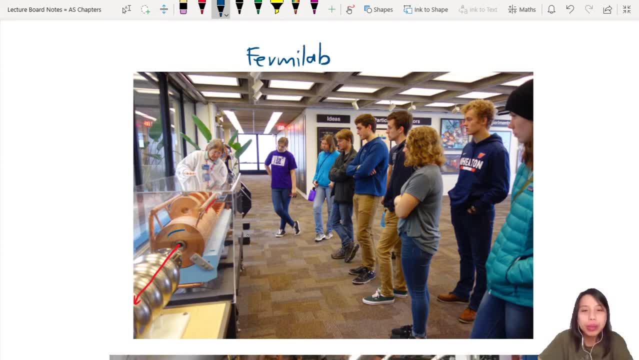 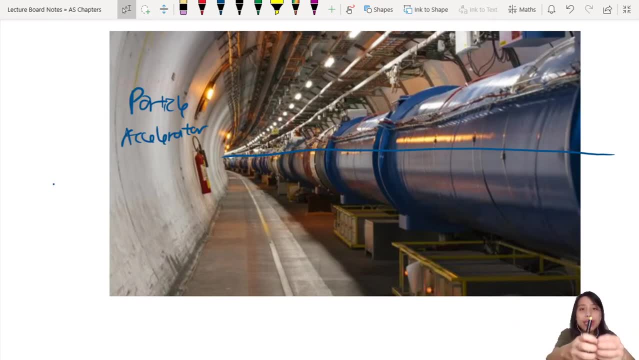 to shoot things together in all these pipes, These chambers, we call them, And of course people discovered stuff. It's like: oh, When you shoot things together, it explodes, The proton explodes, come out, got things. So the proton is not a fundamental particle anymore, Anyway. so 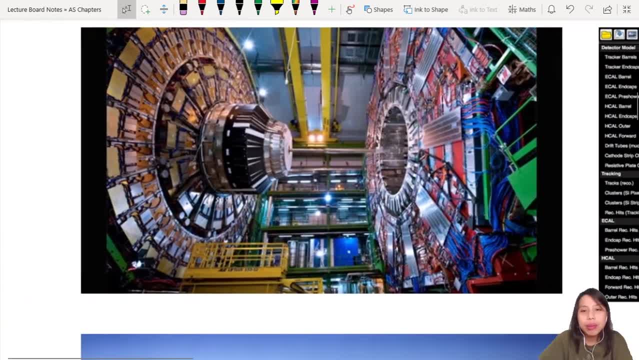 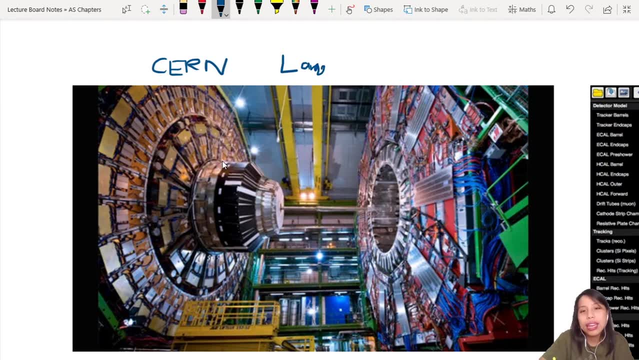 they made it bigger- particle accelerators and they built- I guess it's one of the biggest ones. okay, It's an institution called CERN and this is the Large Hadron Collider. Have you heard of it? No, Okay, Pretty cool stuff. Very amazing discoveries made in the past. 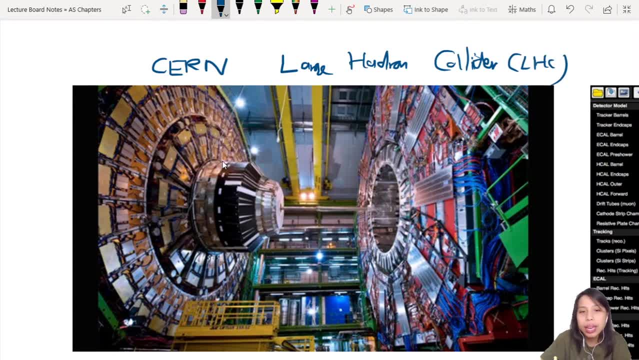 few years LHC. Okay, So a beam particle has come up. It's a big, big, big, big, big, big particle. right, You can see it: One pimple onerat And one particle, two particles. 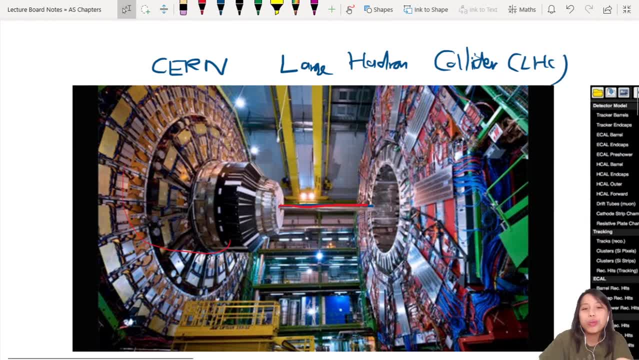 If you look at here, you can see that you guys can see the particles come up and then they smash them together. If you're watching wow, all this big, big stuff, you need a lot of energy to speed up particles, you know. Okay, So what they do is they smash particles. 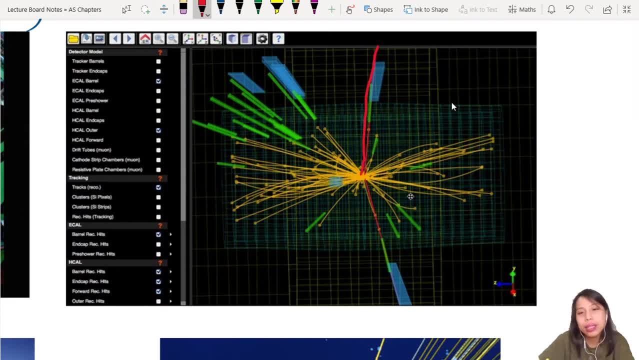 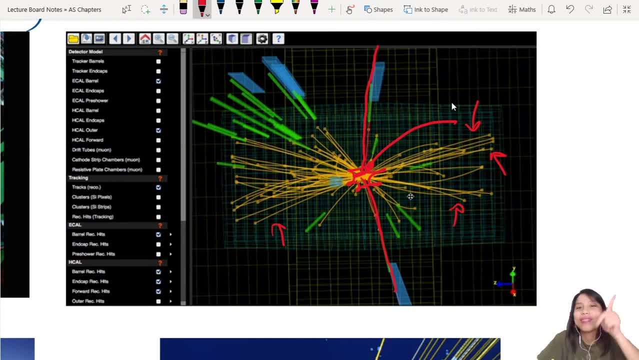 What is this? And depending on how much they deflect- Sigh- they can roughly tell how heavy this particle. and if there's no particle with that mass, then they call a new name. if i want to call it alley particle, it become alley particle. okay, you just create some names. basically, you just smash things together and see what comes out. 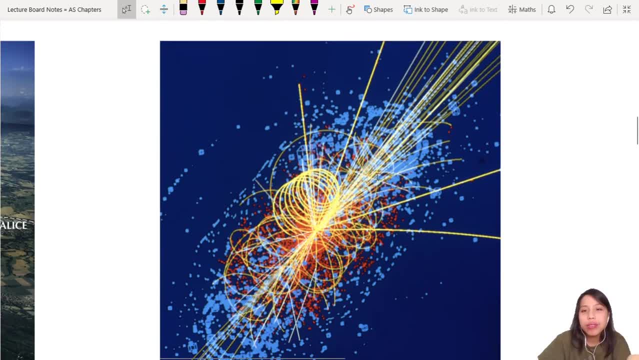 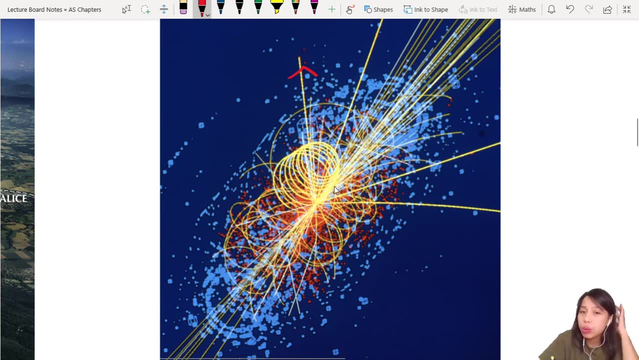 okay, this is a very nice diagram. you will see if you see anything like this. that means particle come out. okay. if it come out straight means no charge, it's just going straight. but you see them do this spiral, spiral thing means that particle probably has some charge- positive, negative, who knows? whatever, that is okay, this is the circle i was talking. 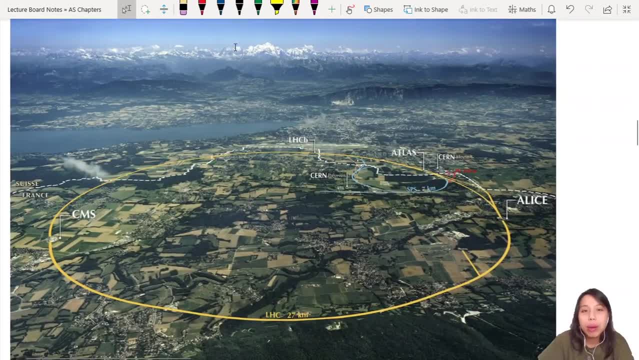 about this is in switzerland. if you ever go to switzerland, you see the mountain in the back. uh, geneva, switzerland is where they have one of the largest experiments. now, okay, that's where cern is at. so you see this yellow ring, right, this is where they will send the particles. 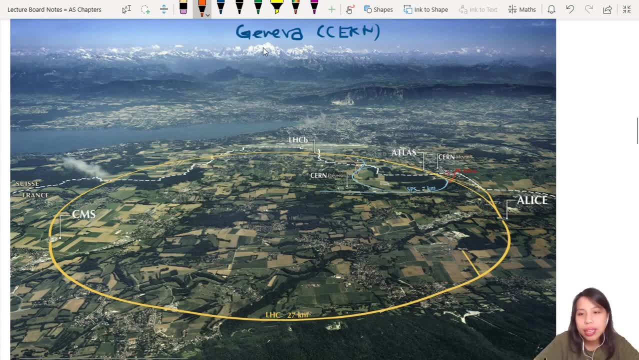 so in one maybe. let's see, let's say, our particle originate from, let's say from here. okay, they will shoot one particle this way, they will shoot one particle this way. then they go around and they collide each other somewhere else. okay, they'll go around many times before colliding. 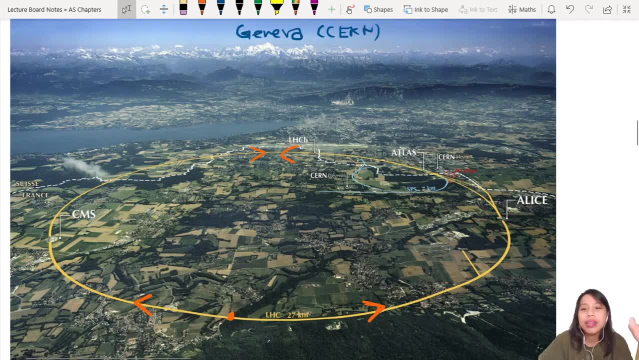 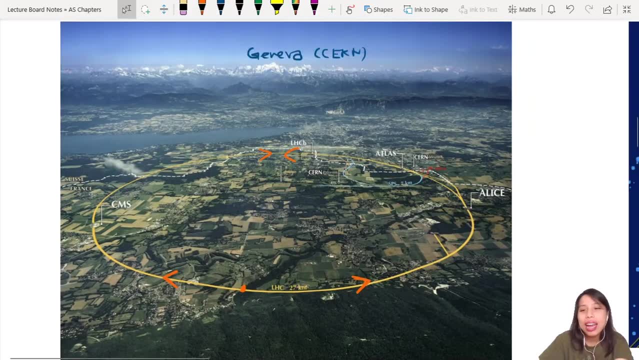 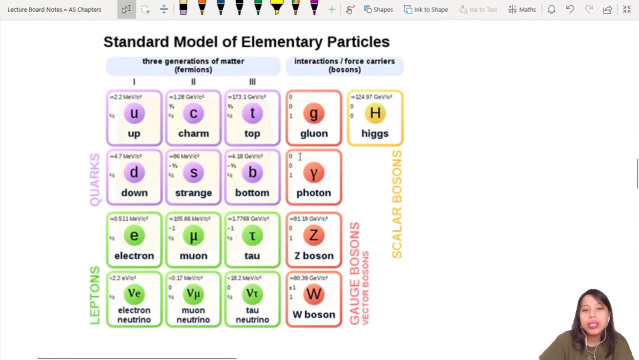 but that's the whole idea why it's so big: it's under many, many cities. welcome to switzerland, home of particle physics- well, current home of particle physics anyway. so they were all happily smashing things together and they discovered lots of stuff. they discovered like, oh my goodness actually got so many, so many particle that is more smaller. 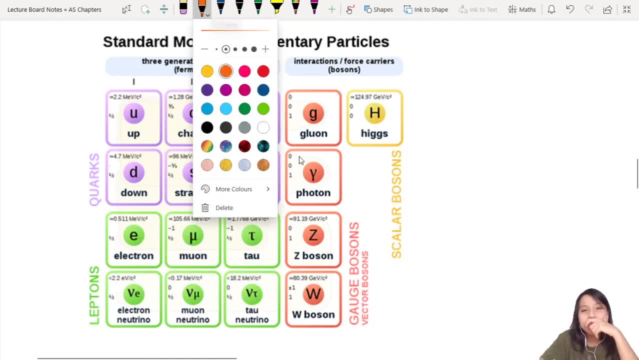 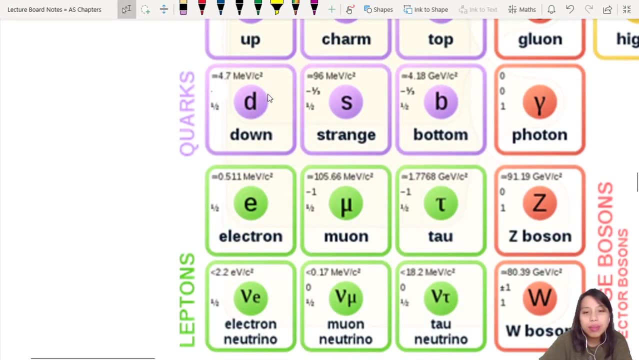 than the proton. okay, um, do you need to memorize all this? well, you need to memorize some important ones, not all of them, okay, the most. the first one that they found. you call this first generation. see the one there. first generation. what did they find? they found, like, oh, up down electron. and electron neutrino. we've seen that work before. so electron are the initially worked first generation. they forget that ever since they find electron neutrino because of the downstream the. so likewise when we look at atom is a particle which we only could use but application or add some evidence so that way, Power. 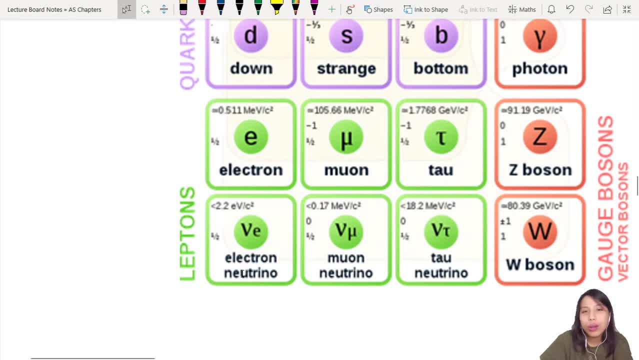 you could比如 we could use people that. it's just part of the material, the ability to do that. once you electron, of course, la electron. we already know that's what I call first generation electron neutrino. they discovered it somehow. we won't go into that. 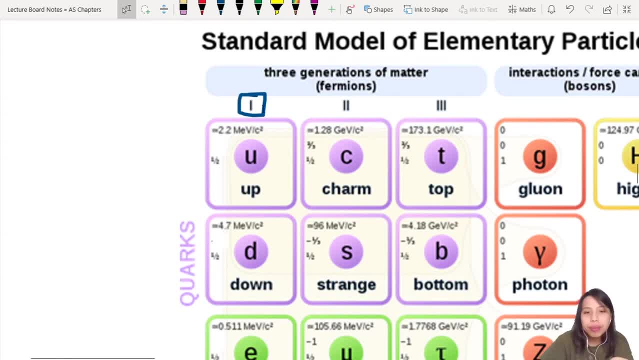 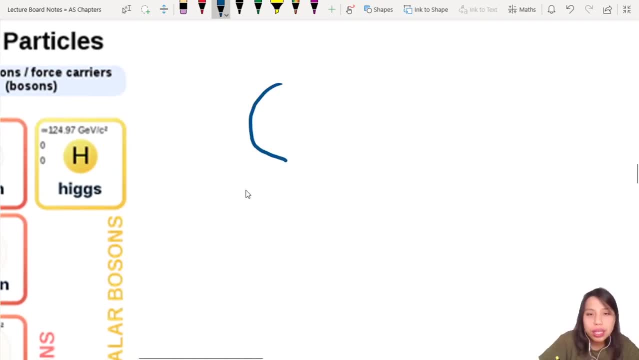 but the new one they found was this: up down fella. what is this up and down? ah, let me draw for you. so when they smash together things, they discovered that, hey, your proton actually is made out of three, what we call quarks: the up quark. 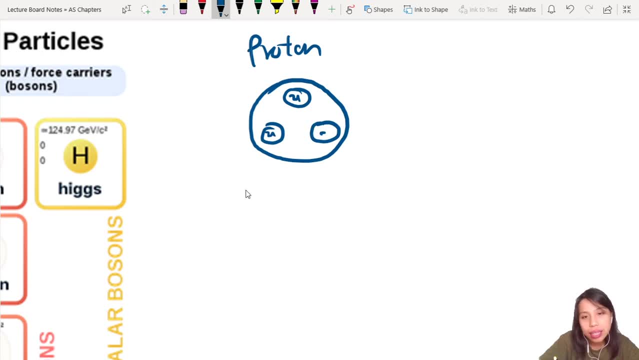 okay, another up quark and a down quark, and then they are all held together by something. somehow they must stay together, ma if they break apart then you don't have proton. so they're like: wah, very magical, what is this? up and down? okay, these are called. 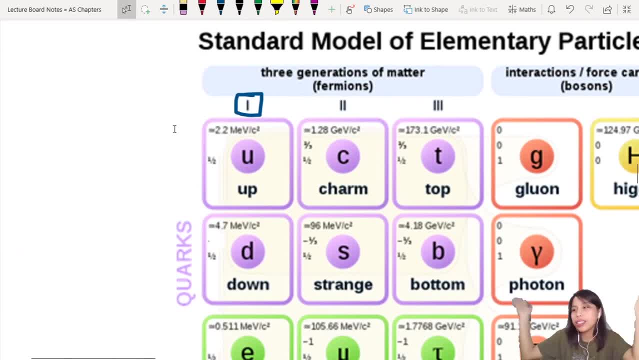 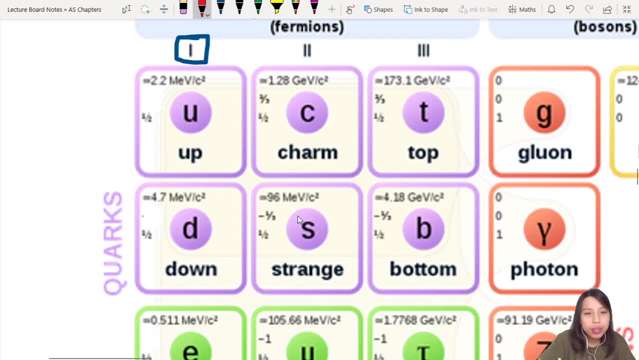 quarks. okay, all this purple color one here is called quarks and each of them have charge. you might want to memorize this one. so the up quark has a charge of plus minus, sorry, plus two over three. e same for the charm and top wah. 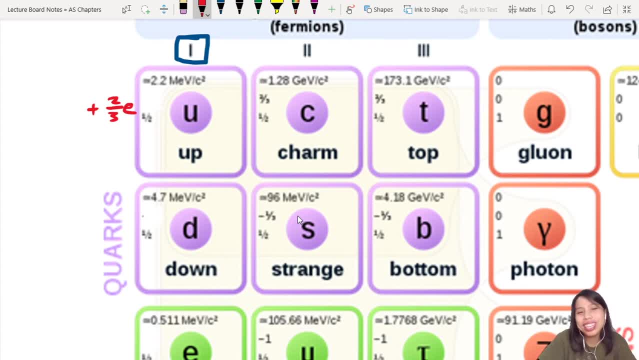 you see the name they choose, very charming, very strange. I still don't know why they choose that. you should ask the person who discovered this one, this one also: two over three e. okay, two over three e. what is e elementary charge? if you're wondering, what is this, 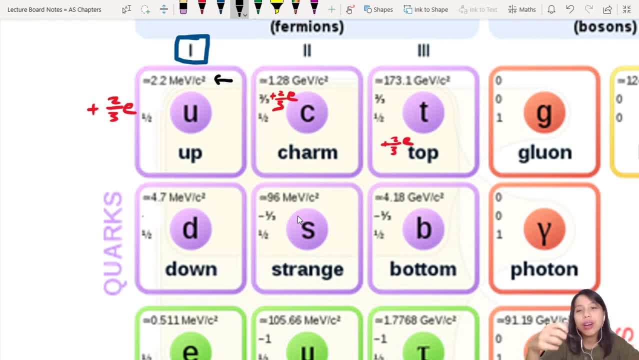 thing here. that is just the mass energy of that quark. okay, see, it's getting bigger and bigger the number. so you need bigger and bigger energy to discover. so up and down were the first one to be discovered. then you build a more powerful particle collider. then you discover. 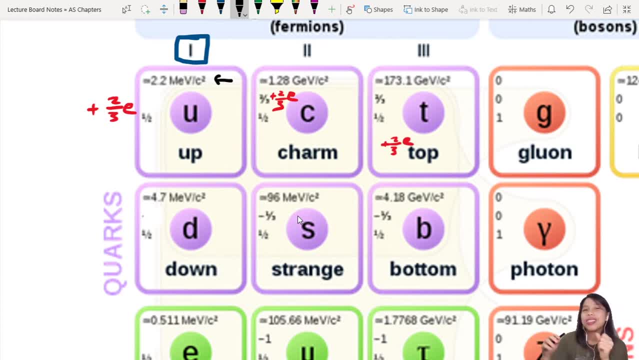 charm and strange, you build another, more powerful one. you, you send these beams at very high energy, collide, then top and bottom come out, but they're very unstable so they sometimes will decay into up and down anyway. so all this across is two over three e down quark. 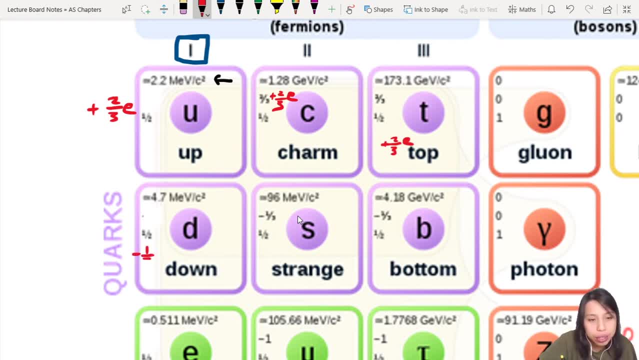 is a different charge, a different charge, electrical charge, like I think of it that way, one over three e also same one over three e. that one you must know, at least for up and down. so memorize those so down, strange and bottom. first generation, second generation, third generation. 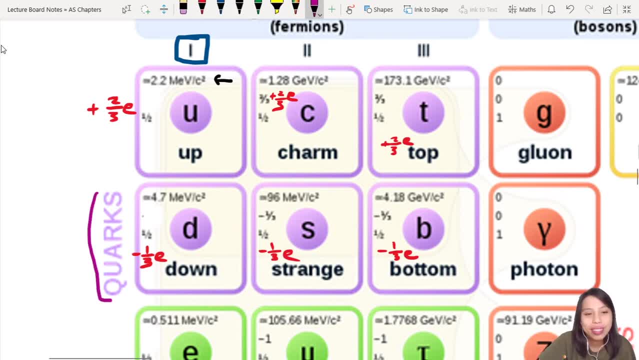 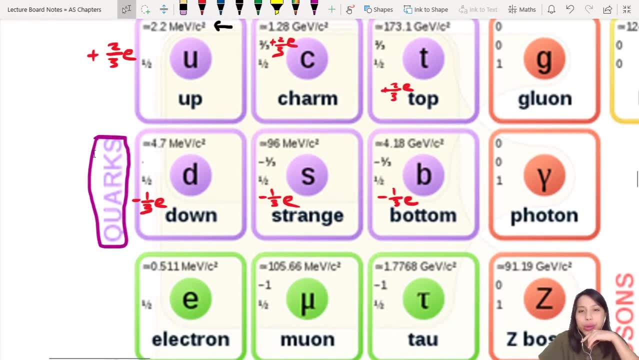 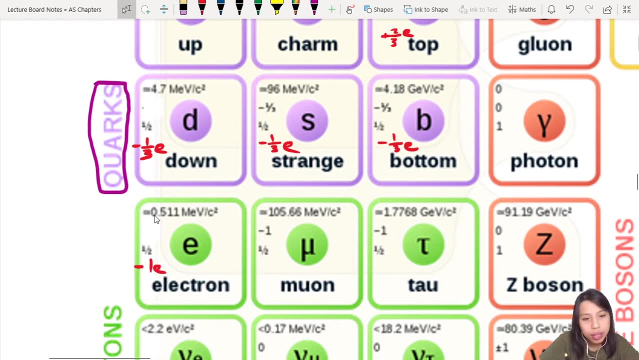 all the purple ones we call quarks, quark, quark, quark, quark, quark. okay, and since we're here, might as well go along with charges: electron. you know what the charge of electron is already, so this is negative one, e same for your mu one. 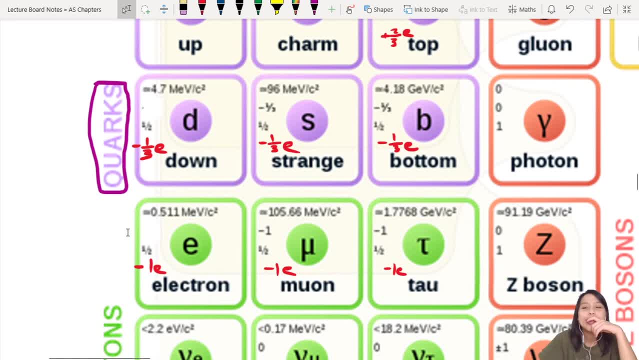 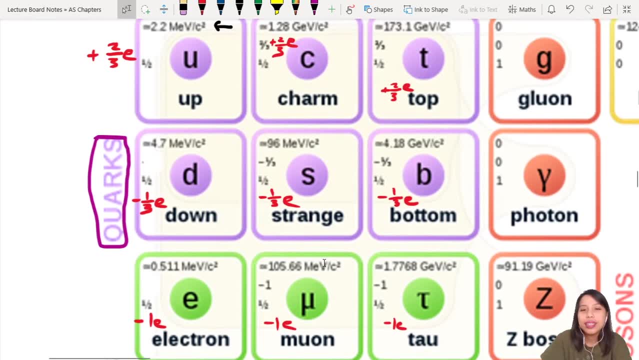 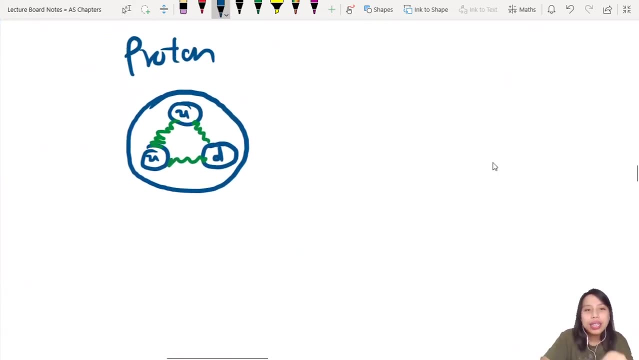 then your tau one, tau, tau one. actually they call it tau one. these are all we call leptons. they're all the green color one. don't worry, we'll have a classification later. okay, so many many particles come out. wow, so back to our proton. how did they come with this conclusion? 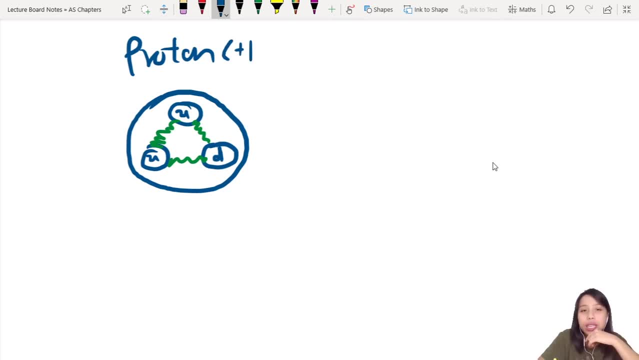 well, they kind of put a few things together. and because we know the protons charge is plus one e right from previous nuclear physics. so if you have a proton made of up, up and down quark, up and down, quark, up and down, quark, that means oh. 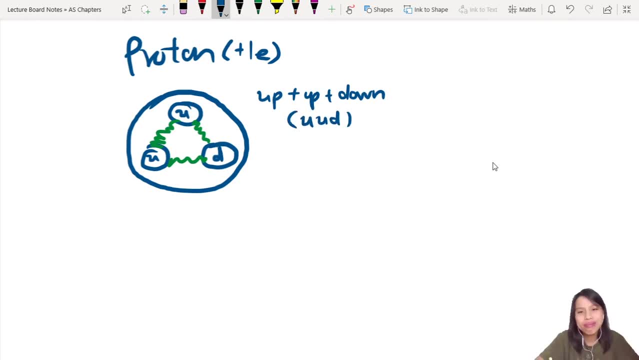 oh, by the way, we can say this uud up, up, down, lazy to write everything. so that means the total charge. what is the up up is- just now we said it, ma- is a two over three up again, two over three plus. what's the charge of charge of this down? 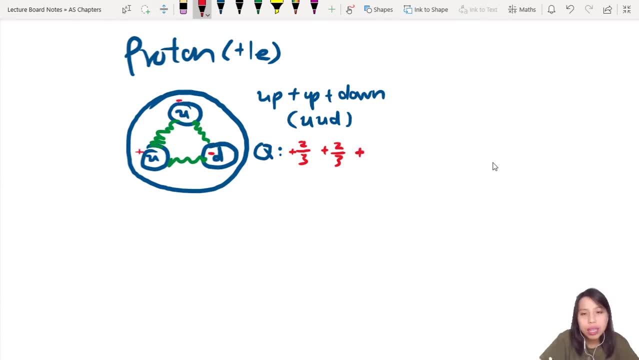 it's a negative, it's a positive, positive. down is negative, one over three. so you add together what you get. so then the charge of a proton should be: so then the charge of a proton should be: what is two over three plus two over three, plus one over three. one e, though. so 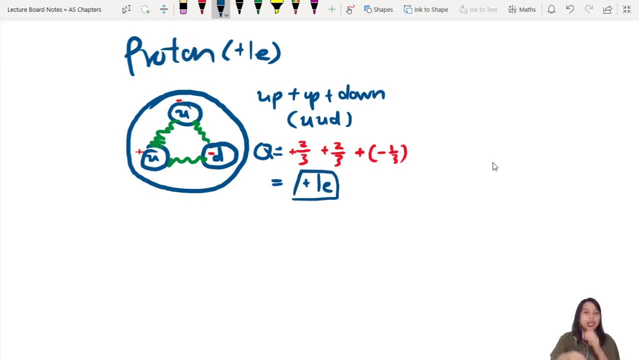 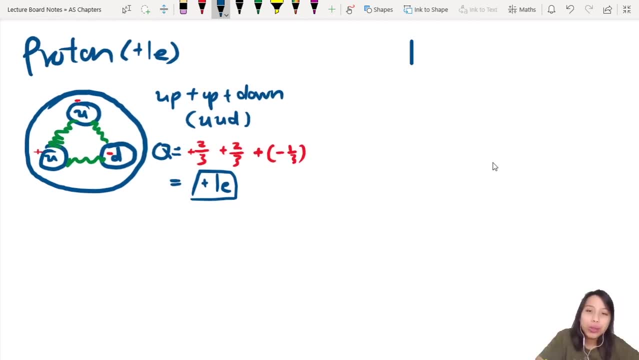 plus one, e that's how everything fit together. they're like: oh, yes, yes, yes, this is how we can put things together. not only they broke down the proton, they also found out neutron actually can break down into quarks. neutron is zero charge, right, so neutron, let's say you have. 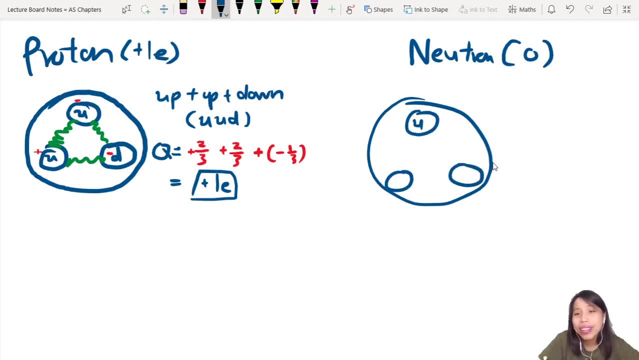 one, two, three. you will take a guess. it's made out of what. how do you get a zero charge? you need a up. okay, because up will be two over three. uh, what else you need? cannot add some more? okay, i'll try down and down. so down and down. so this will be udd. 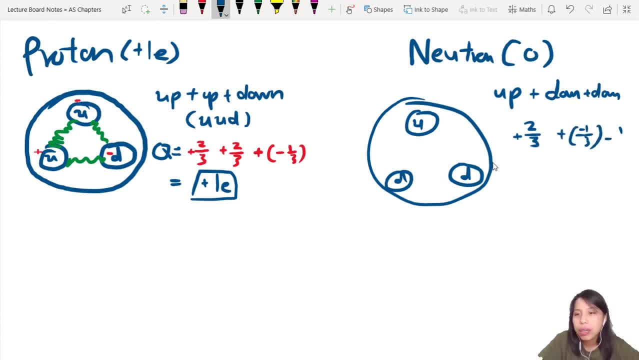 plus negative one over three. actually i just write minus minus one over three, so this one will give you zero charge. that's how we know that is made out of up quark and two down quarks. okay, this is q the charge again. somehow, all these quarks are. 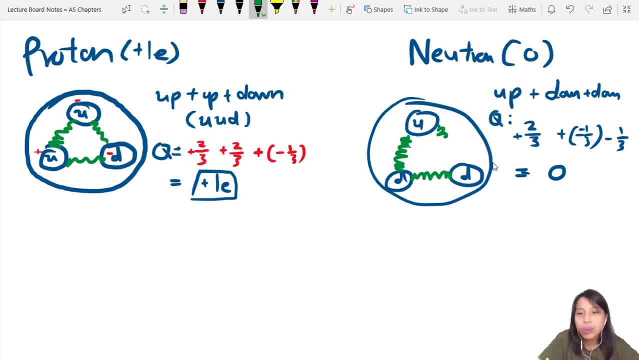 staying together. i don't know what to draw, so i draw a spring kind of thing to say like, oh, there's some kind of thing holding them together. but then, if you want to think about it, what actually is holding these things together? we come up with some names for. 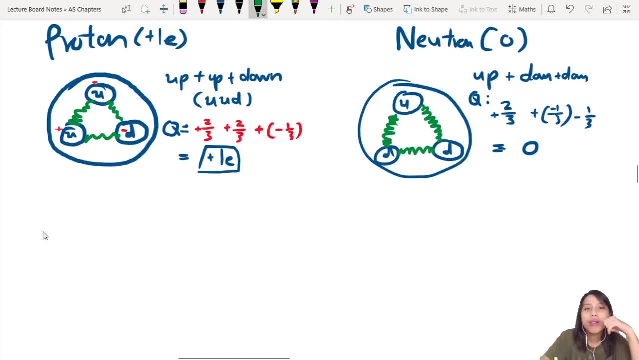 it already. okay, these are what we call the four fundamental uh forces of the universe. okay, can you take a guess what they are? think about it. see what are the fundamental forces. don't say like tension, normal forces, no, no, no. fundamental forces of the universe. you can think of it this way. number one: 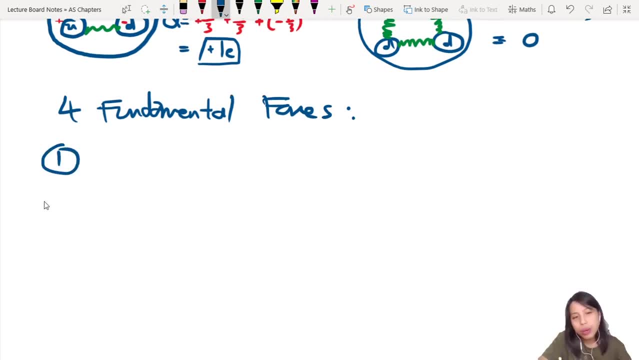 the first one, ding ding, is what we call the strong nuclear force. oh, what is this? this is the force that acts uh, on quarks- oops, i should say x on quarks and anti-quarks- empty, i have no space there. okay, i put like that: quarks or anti. 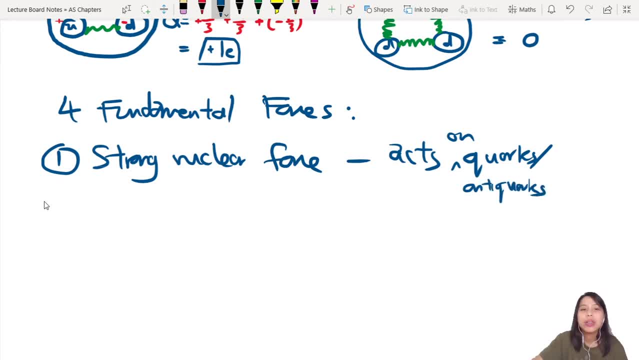 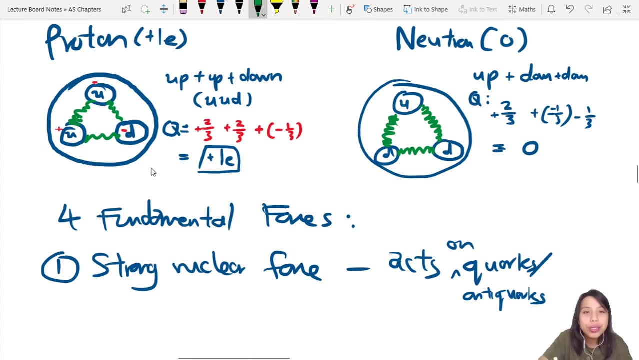 quarks. so you see the green color spring thing that i draw right. this one, this one, that is your fundamental force, radio strong nuclear force. okay, let me draw a line here. so this is our strong nuclear force that holds them together, okay? um yeah, i'm wondering like what? 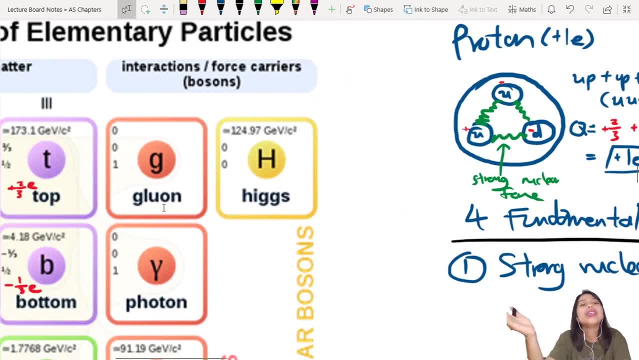 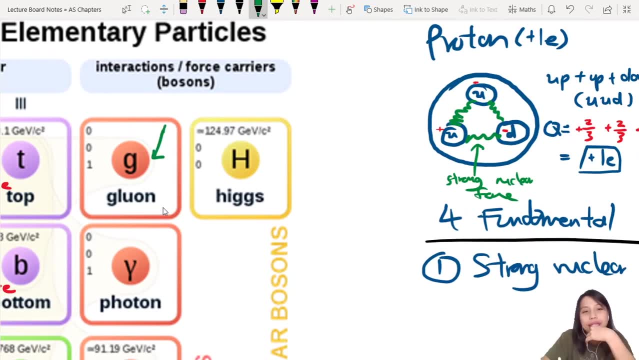 why got a what? what is this? to be honest, we don't really know, but we do know it's related somehow to your. maybe your glue on? ah, okay, this one will help you hold things together. so you're up and up actually throwing glue on each other. 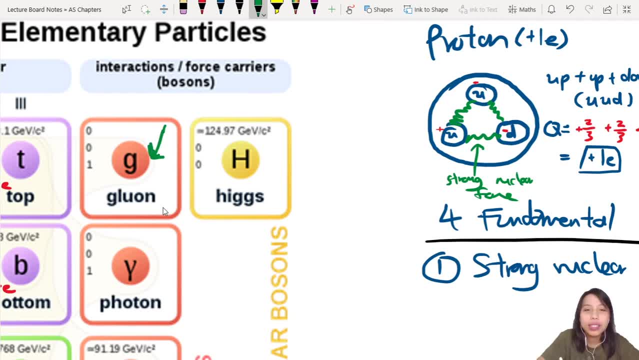 and creates a force. so how does it actually relate? go and search out some videos. okay, so there's some related to strong nuclear force. these are all bosons, by the way, called force carriers, so these particles carry force. wow, how does a particle carry force? mind blowing, very hard to bring, it's okay. 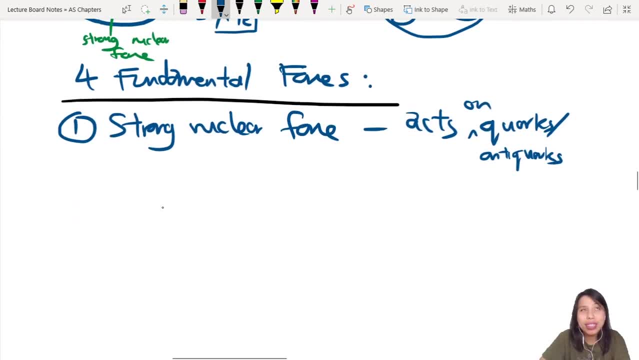 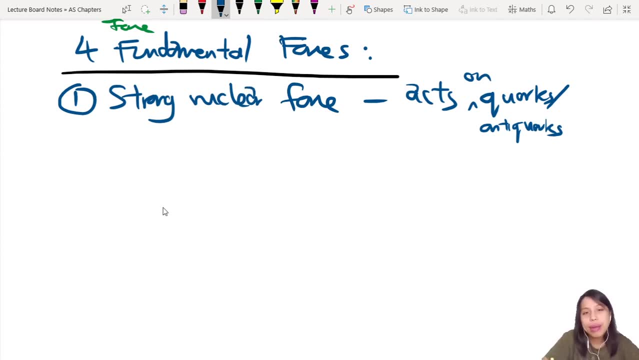 we just, we just we just discovered this in the last like 10, 20, 30 years, so it's very new physics for everyone, okay, uh, what else? okay, so this one force- you just need to know the name, la, okay, and roughly what it acts on. 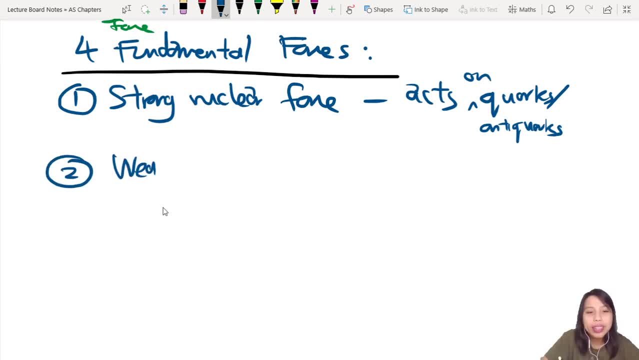 another force. got strong, ah, means got weak. no, okay, also weak nuclear force. they don't know what to call it. what is a weak nuclear force? it acts on all fundamental particles, ah, all the interaction between fundamental particles. so all fundamental particles. so all fundamental particles means all. 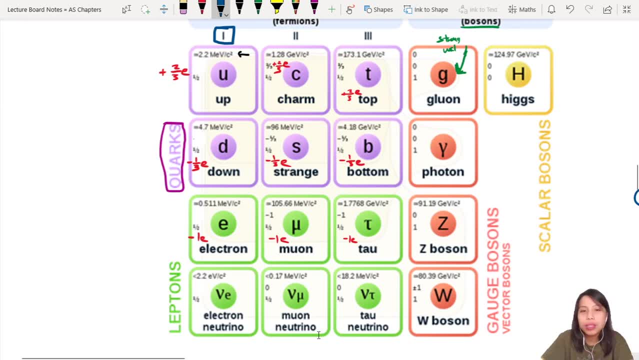 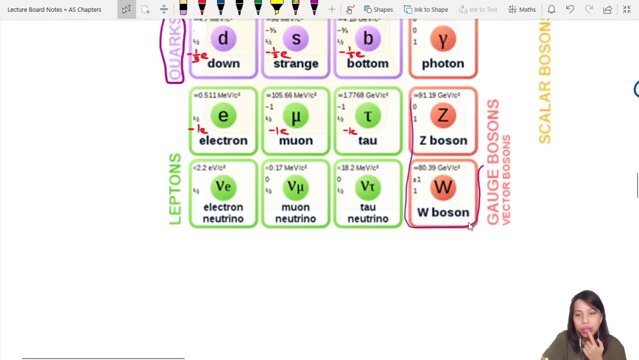 of these law, all the quarks, all the leptons, when they interact with each other. you have some kind of weak nuclear force there and your weak nuclear force is- well, you can say it's mainly related to these ones- la bosons, the w and the z. 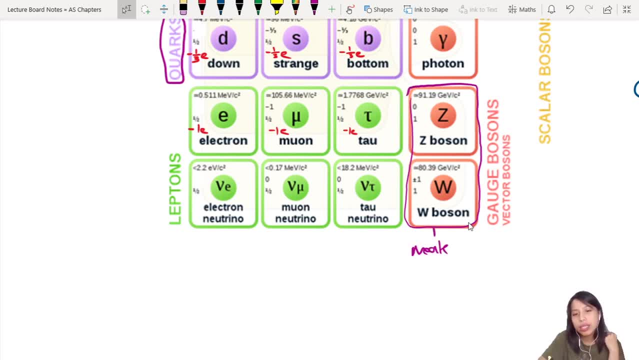 they don't know what to call it. so w and z. a lot of them, a lot of the interactions are from this w and z. okay, all right here, mainly for interaction with nuclear force. so if i throw a w at you, you throw a w at me. oh, 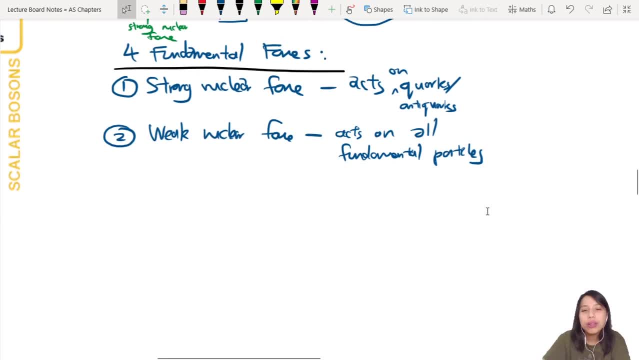 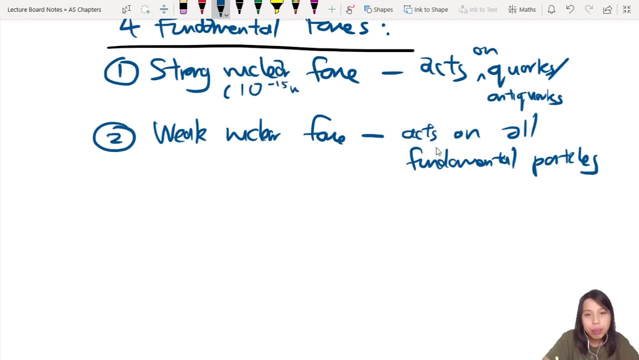 got interaction any long, weak interaction, okay, and these are on a very small scale. what do i mean by small scale means if you are 10 to the negative 15 meters away, then that is roughly the how far the scale of the force can be, la. if you're further away, then you cannot. 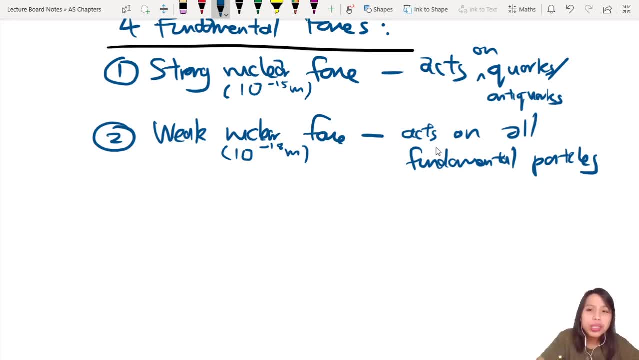 really your quark here, quark, there cannot. okay, uh, two more forces. try and guess what are the other two forces, fundamental forces? i know the first two are a bit new to us, but what's number three and number four? number three is actually what we call. 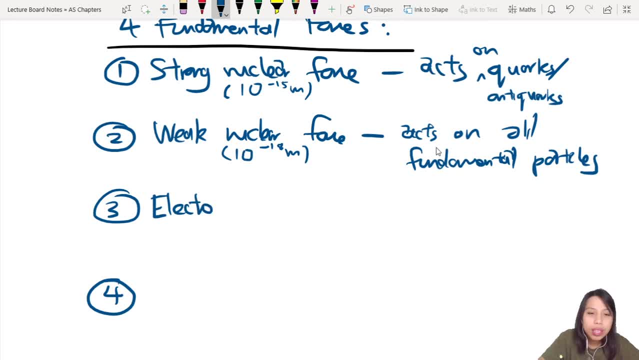 the electromagnetic force, electro magnetic, if you're wondering, is this related to electric force? that we learned in electric field? yes, but also got magnetic, ma you see electro magnetic. so electric magnetic field sounds like electromagnetic wave, maybe some related. okay, this one mainly acts on charged particles, because you must have charged, okay. 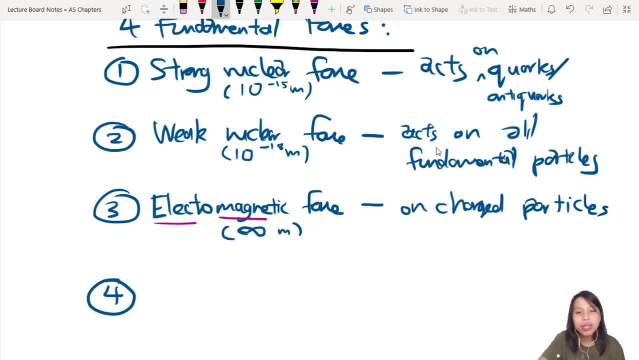 and this is actually the range is very big: infinity meter. if you are here and you are in the next galaxy, there's some kind of interaction also. so as long as you got charged up, so that's what we call the electromagnetic force, okay, sometimes related to the photons- 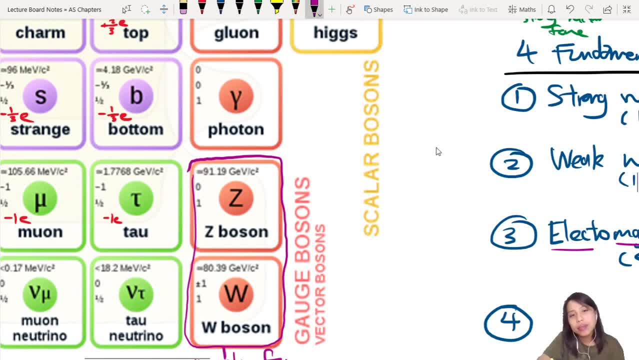 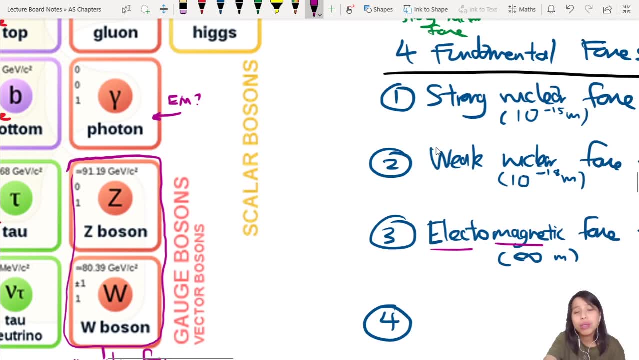 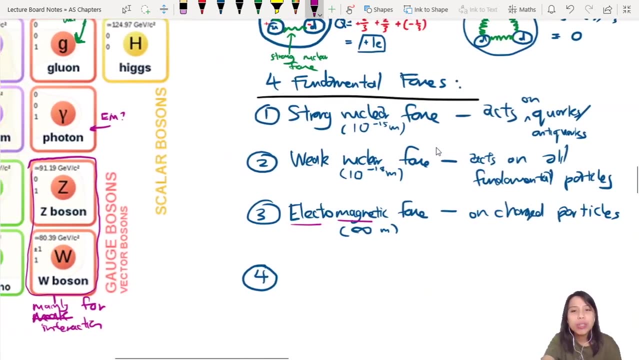 people suspect: okay, um, em question mark. okay, i'll put a question mark there for you to study more if you want to, but not if you don't. it's okay. you don't need to know that at a levels, uh, last force, almost there, almost there, uh, can you, can you think of a? 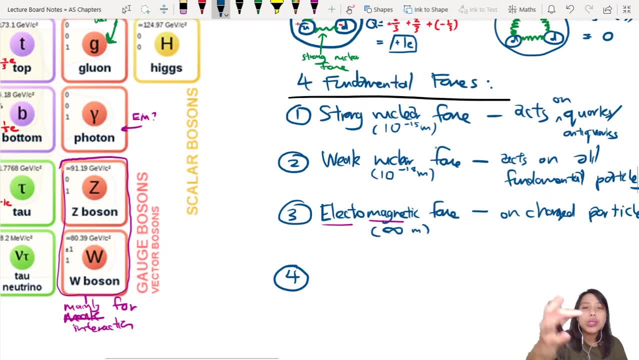 fundamental force, the one that is crucial to our existence. well, that's called the fundamental force, the um, gravitational force, or gravity. you know, i'm just gonna put gravity or fg. so gravity is actually a fundamental force that we did not really know how to think of until quite recently. 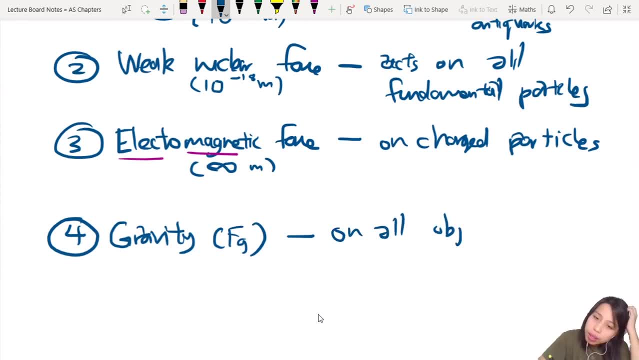 of course gravity acts on all objects, say objects, that has mass. but then even we realize, actually, you know mars also kind of affected by gravity, or question mark. okay, so a lot of new things. we don't know, don't know, don't know. this is like the 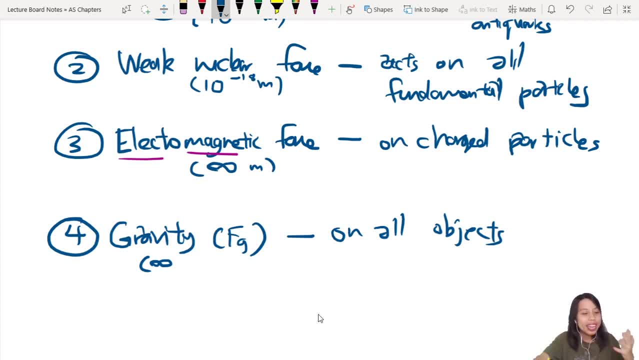 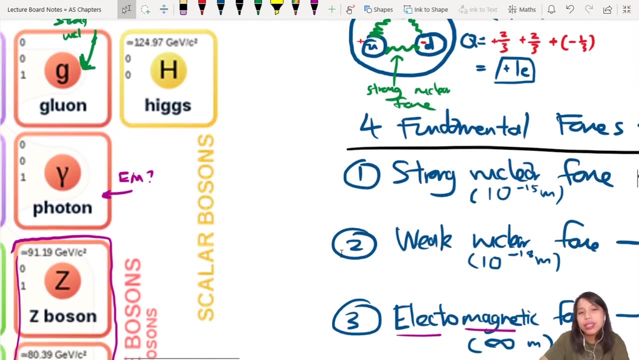 this is at the edge of our knowledge. ready la, okay, we're at the edge of scientific knowledge. uh, it ranges infinity meter, very far away. you still can have gravitational force acting on you. okay, um, and very, very, quite recently we discovered- not we, la scientists, humanity discovered- 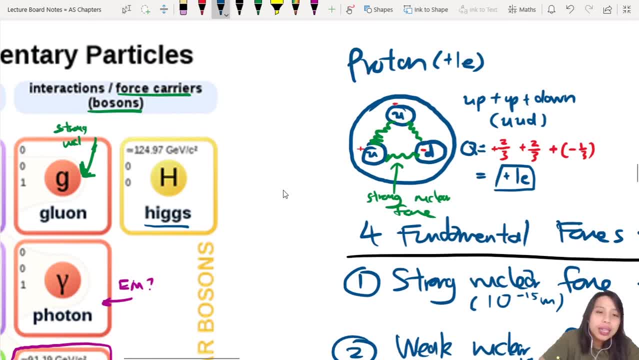 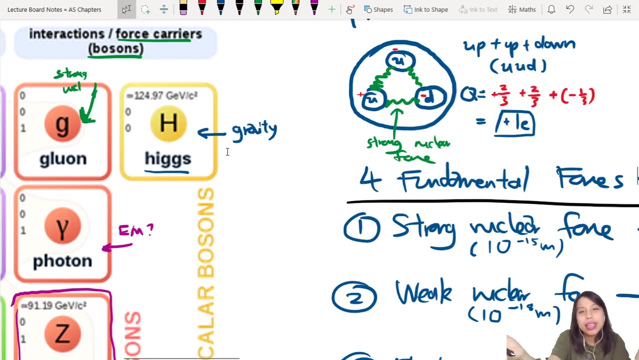 this thing called the higgs boson. this higgs, they discovered, is related to the gravitational force. why do we have gravity? why do we have ma mass? why, what, what, what? so if something is acting on you, a gravitational force acting on you, that's because that thing is throwing. 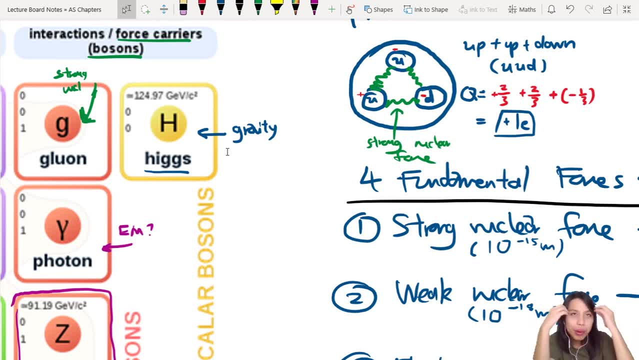 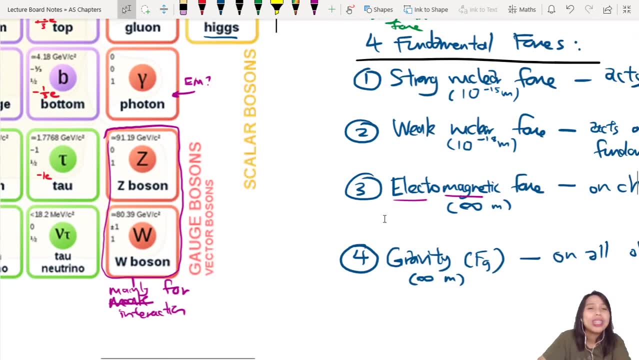 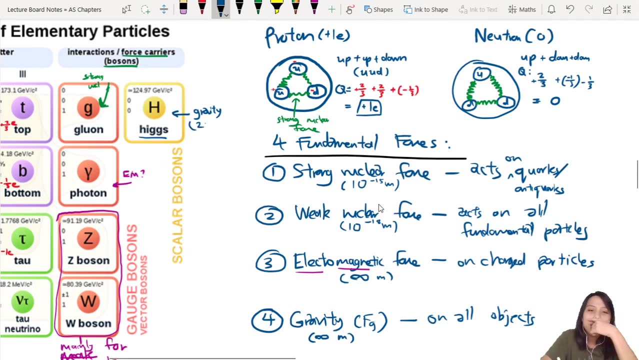 higgs boson at you, so it's interacting with you. oh, mind blown, this higgs boson is a force carrier that is the one that causes our gravity. so if you want to learn more about this again, go and google it. plenty of information. pretty recent discovery, i think 2008. 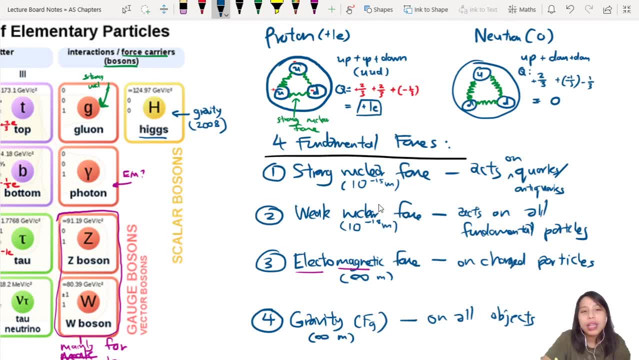 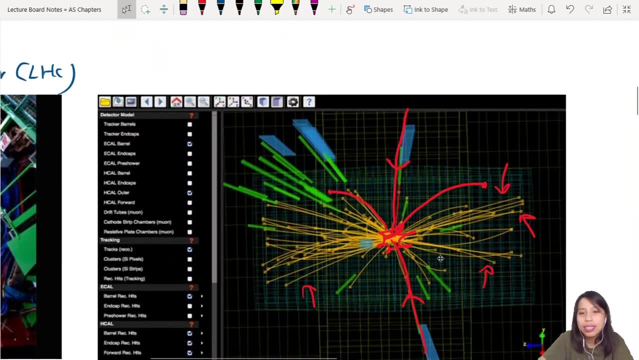 okay, forgot already. go and check out. it's about 2008. they won a nobel prize for discovering the higgs boson. just by looking at diagrams like this and like this and they tell, oh, higgs boson. and then they go and make theory: la, everything okay so. 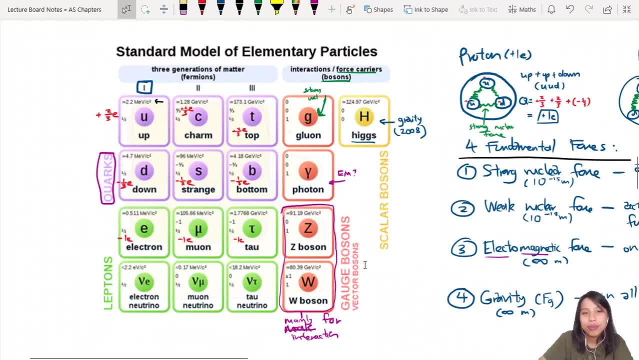 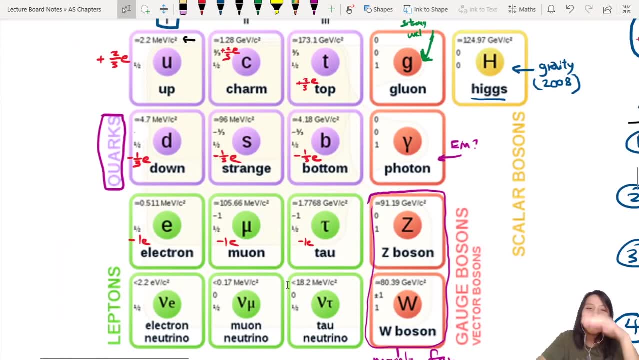 this is our zoo of fundamental particles, quite fascinating. a lot of them, okay. and because there are so many, or eventually we scratch our heads and we like we need a way to classify all those. that's why we come up with these names: leptons, quarks, but then there are more. 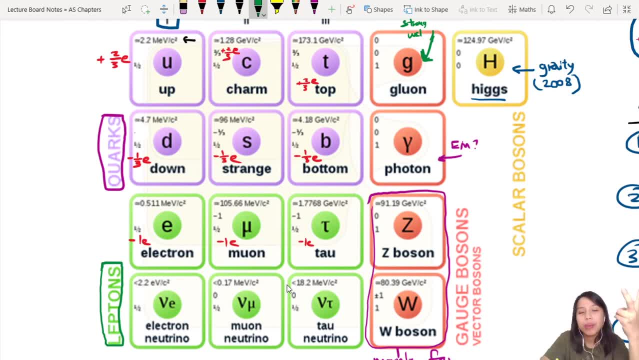 ways to classify these types. so there are two types. here are two primary types. okay, you look at the purple one quarks, the green ones leptons, and then you put all these together in different combination, or then you get proton, neutron and so many, so many different particles that people 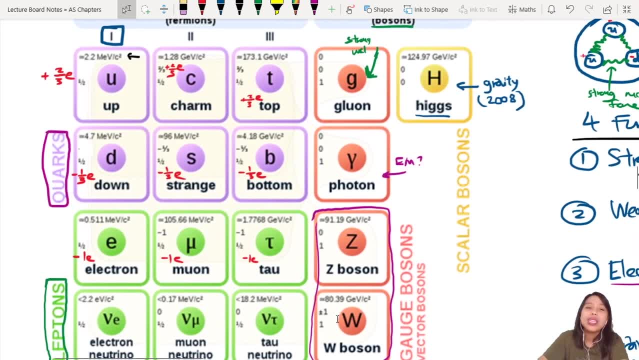 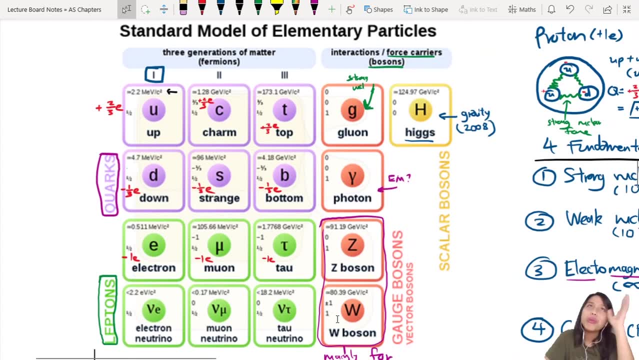 decided: okay, hot stop, we need to come up with a classification system. classification system, you want classification system. it's like you know, in biology we like: oh, human is what genome is what phylum is what kingdom, animal kingdom, plant kingdom- got backbone, no backbone, so they draw a. 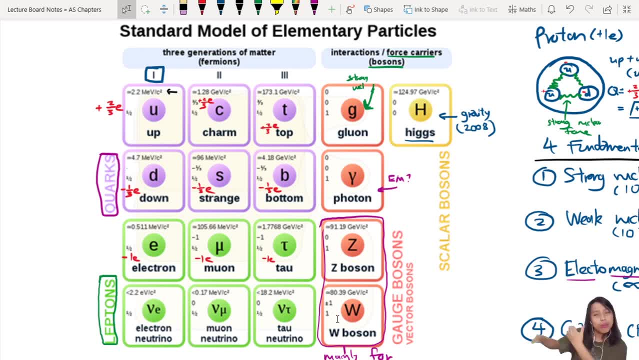 whole classification system for animals and you know life. so we do the same thing for particles, okay. chemistry has the same thing, group one, group two, group three. this one is what type of metal? that one alkali, blah, blah, blah. we do the same thing with particles, okay. 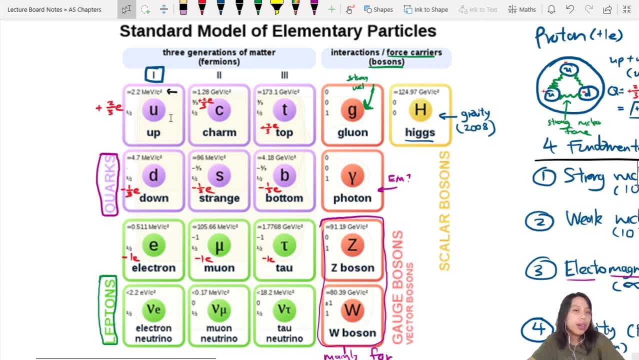 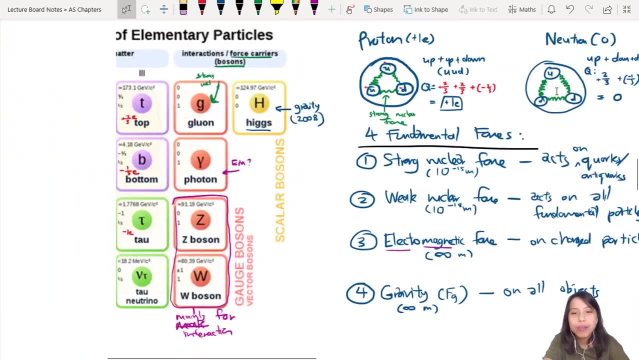 so let's go and see: uh, how can you classify all these particles and fundamental particles and make more sense out of them? okay, so let's go take a look at that.